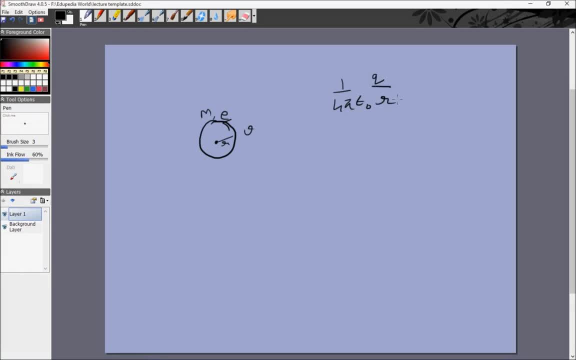 this: q by r squared is equal to mv squared by r Right. this is the standard Bohr model. We'll study it in much, much detail when we reach modern physics. that is, much, much later in the course. but this formula is quite easy to understand. Sorry, this should be kqe. 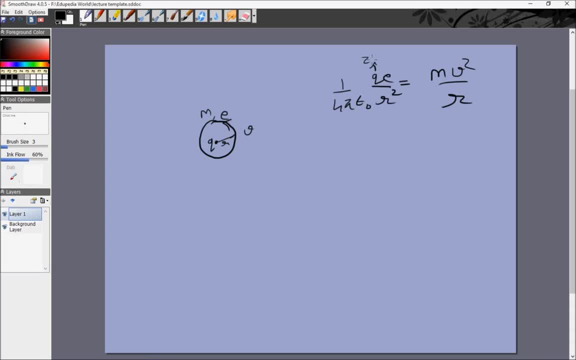 q is the charge on this. q is sometimes written as ze. z is the atomic number, number of protons, and that multiplied by e is the charge here. Anyway, that is not important right now. Right now, what is important is that the electron 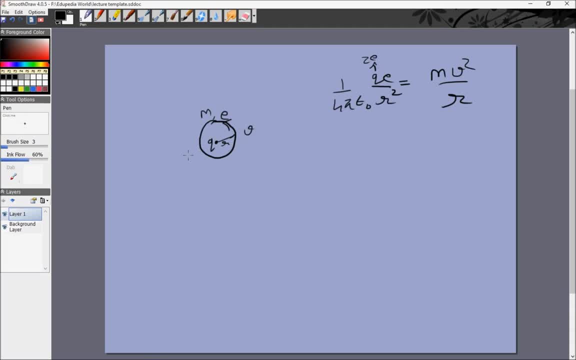 moves with a constant speed, v in a circle of radius r Right. so what is the angular momentum of the electron? The angular momentum is i omega, and that is equal to m r squared omega. Omega can be written as v by r or mvr. 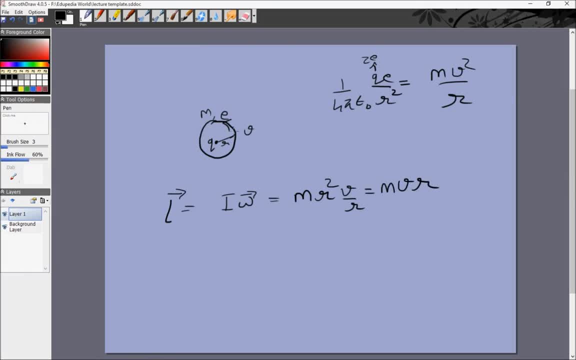 What is the direction, Since this is the, if you curl your fingers along the direction of the motion, then your thumb is going to point towards you, so the direction will be towards the viewer Right. what is the magnetic moment of this loop? After all, an electron moving in a circle. 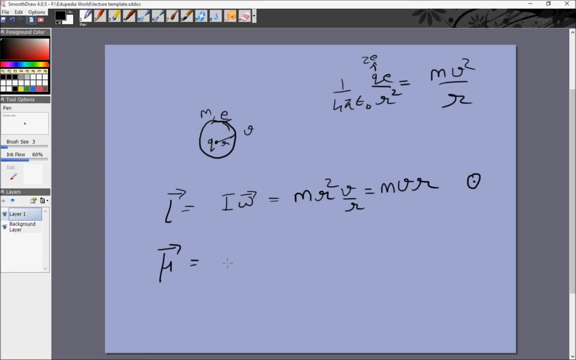 classifies as a current carrying loop. So this is equal to the current multiplied by the area vector right, which is. so first I'll write the area vector. that is easy. that is pi? r squared right, and the direction of it would actually be. 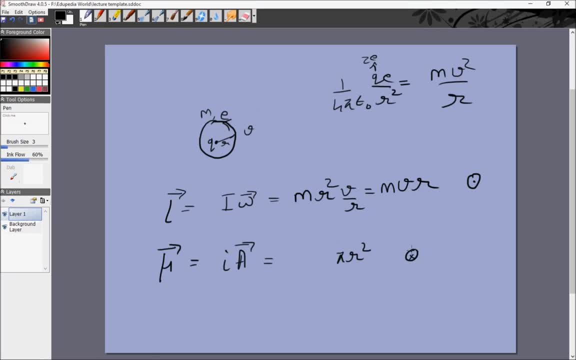 inside the plane. It would be outside the plane except for the fact that it's an electron, which is a negatively charged particle. so if an electron is going in this direction, that means the current is actually flowing in this direction, right? so this is important. So the direction of the magnetic moment would be away from. 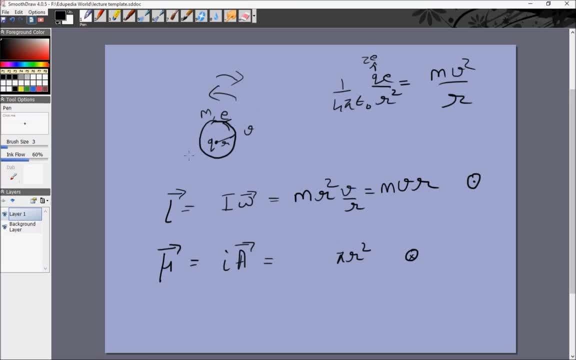 the viewer going inside the plane and the current would be delta q by delta t, the charge flowing per unit time. the charge flowing per unit time period is e, so it can be written as d This: if t is the time period of revolution, then 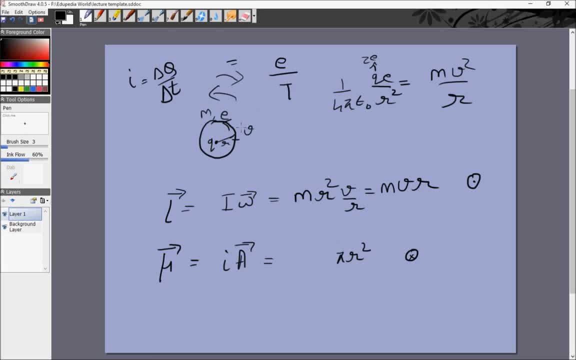 after every time period through any area an amount E of charge is flowing. T can be written obviously as 2 pi R by V and from that I get e V by 2 pi R. so e V by 2 pi R. pi pi cancels R and RS cancel and it comes out to be e V R by 2 coming. 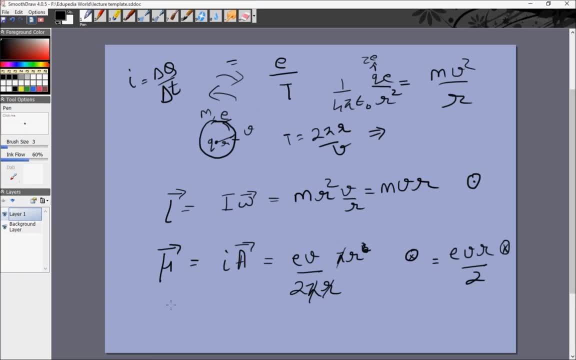 out of the plane. now, the ratio of these two things is a very specific, important quantity: mu by L, and if you look at this, VR, VR will cancel and it will be equal to minus e by 2m, right minus, because they're in the opposite direction. this: 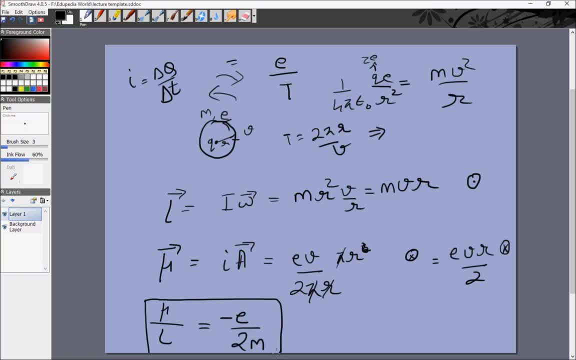 is actually called the gyromagnetic ratio, and in advanced physics this is a very important quantity, and the interesting thing about it is every single particle in nature happens to follow this equation, with some small changes, some of them, it's it's e by M instead of e by 2m, for again reasons. 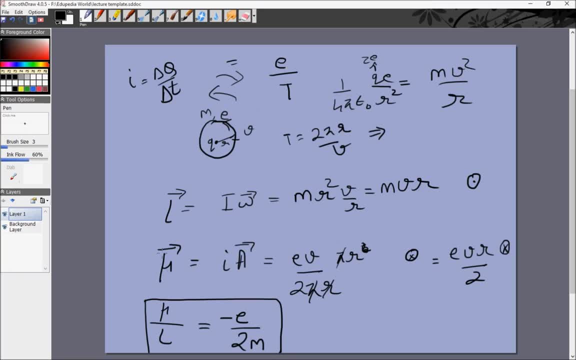 which are not in your course, but this: the ratio of the magnetic magnitude of the magnetic force is equal to the magnitude of the magnetic force, is equal to the magnitude of the magnetic force and the magnetic force is equal to the angular momentum is always a con. E is a constant and M is a constant right. 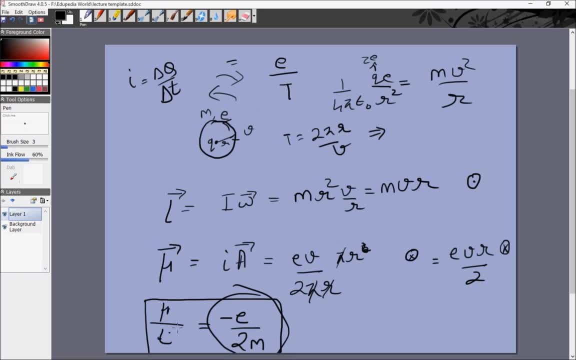 mass and charge, so that these, the ratio of these two things, in advanced physics seems to be a very important quantity, and it is called the gyromagnetic ratio. anyway, for this course, all you need to know is that the magnetic moment is e, VR by 2. that is what is important, right? so now let's see what happens when we 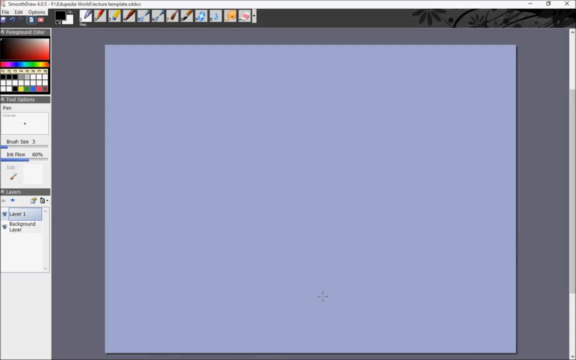 actually put a certain number of particles in the magnetic force and then put a certain amount of material within a magnetic field. so every material is made up of atoms and molecules which are in turn made up of electrons which move in loops, right circles of spheres. so we can visualize all these material in 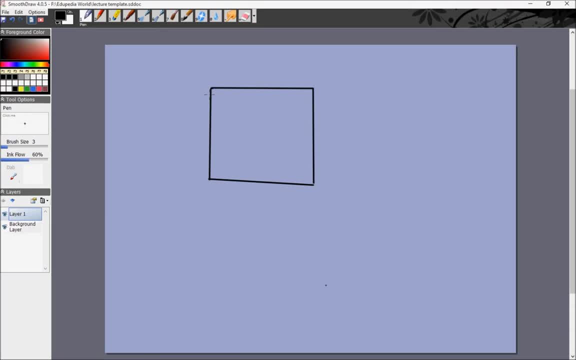 terms of current carrying loops. that is, they might have some intrinsic magnetic moment and we know that the torque on a magnetic, on a magnetic dipole, is equal to mu cross B and it is 0 when mu is parallel to B. so if there are a lot of magnetic dipoles and we apply a magnetic field in 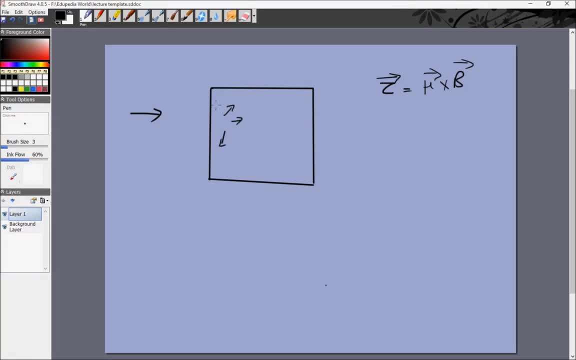 this direction. that magnetic field will end up rotating, all these dipoles in the direction of the magnetic field. in some cases they fetching, in other cases they might not align perfectly, but in any case there will be some changes within these magnetic moments due to these magnetic field, and what will happen is: 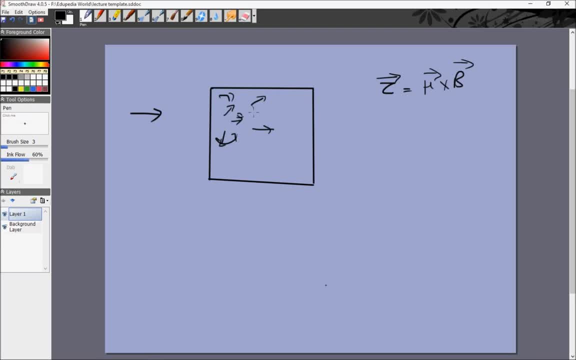 because most magnetic moments, even if all of them are not soiled, they will be shifted somewhat towards E겠어 the right and that will create a net magnetic moment towards the right right. this is similar to if we have a material in which we have a lot of dipoles and 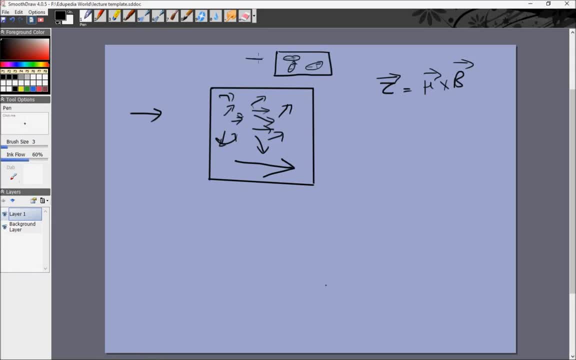 they're in different directions and you apply an electric field, they'll all tend to go parallel to the electric field. but only perfect conductors will completely be able to cancel this, that is, completely be aligned. parallel to this, all other materials will be what is called partially aligned. so even if 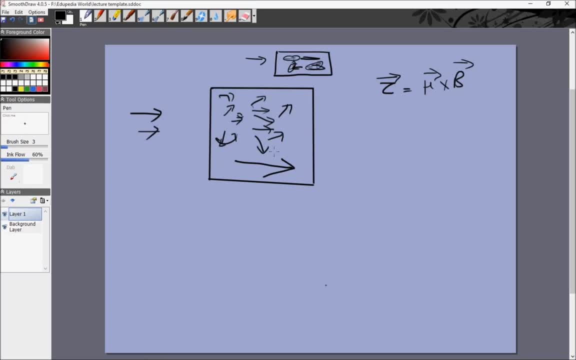 these current carrying loops are partially aligned in this direction. that will result in a net magnetic moment in this direction and an important quantity which is called I, the magnetization. the magnetization is nothing but the magnetic moment. by the way, magnetic moment, magnetic dipole moment is the. 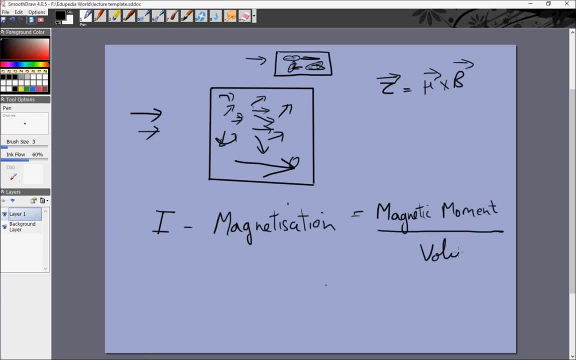 same thing per unit volume. so it is the analog of P, which is the magnetic dipole moment. which is the magnetic dipole moment was the electric polarization right, the direction is my, the direction of magnetic moment. so what was the electric polarization capital? P, that was the 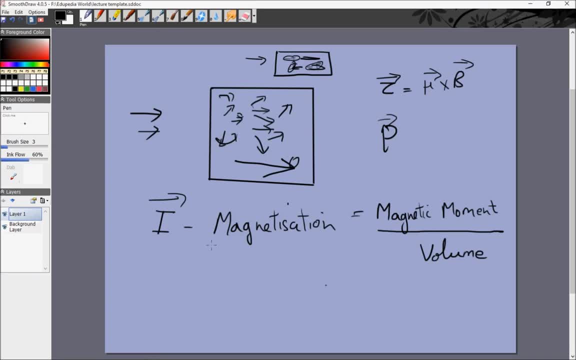 dipole moment per unit volume right. similarly, the magnetization is the analog in magnet statics and that is the magnetic moment per unit volume. and just like for the case of a standard parallel plate capacitor, if this was plus and this is minus, the area is a, this is D, the charge is Q. in that case, P was Q. 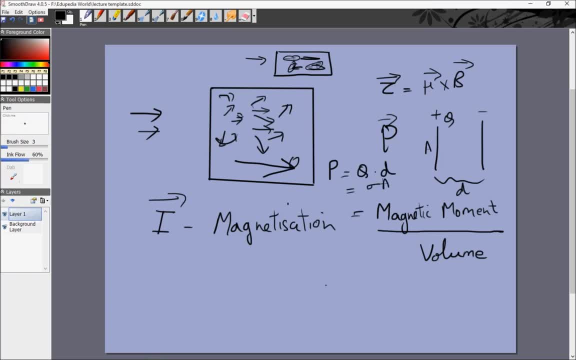 times D, which can be written as Sigma ad. so P by ad, that is, the volume was equal to Sigma. that means the polarization was equal to the surface charge density. similarly we have a relationship in bar magnets for magnetization and pole strength. if this is a standard bar magnet, then this is minus M. let's say: 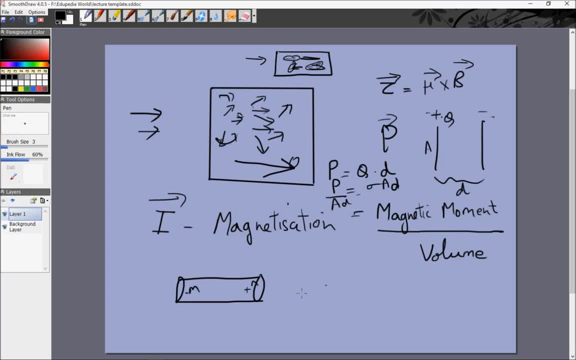 and this is plus M, the magnetic moment is 2 ml right and the magnetic moment divided by volume, if this is total, is 2l and the area is a 2l times a, or that is M by a. so the magnetization for a bar magnet is simply the pole strength per. 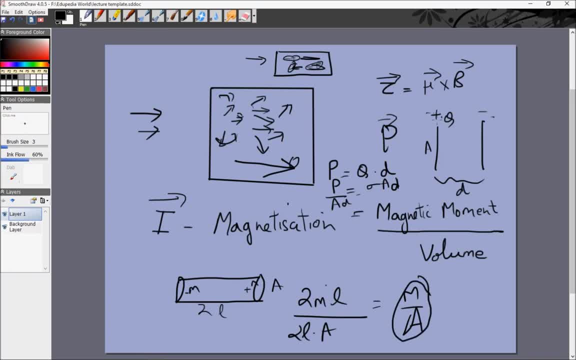 unit area. just like the polarization was simply the charge per unit area or charge density in the case of a capacitor, so again we keep seeing this analog and parallels between electricity and magnetism, which is quite nice, because you only really need to remember one of them and the other one can come. 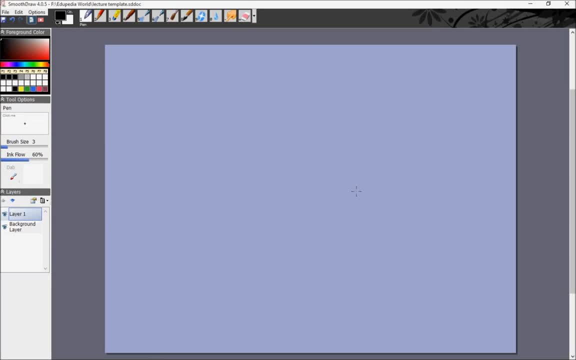 pretty naturally. now let's look at what happens in when we put any material in a magnetic field. now there are many three different processes which might happen depending on the type of material. but there is a particular process, one of the three, which is called diamagnetism, and it is present in all materials. now the other. 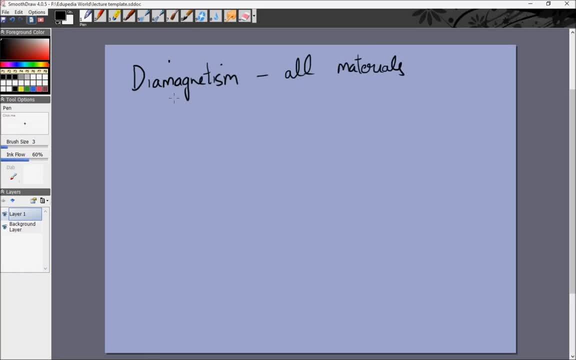 two processes we will study are paramagnetism and ferromagnetism, and some materials exhibit those and the materials which exhibit paramagnetism and ferromagnetism generally. the magnitude of those phenomena is much greater than the diamagnetism, so end up, they end up overshadowing the diamagnetism right. so 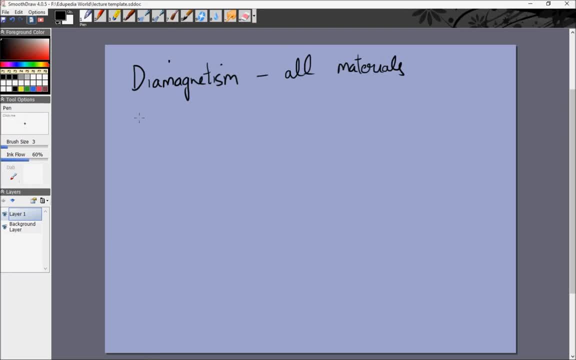 students sometimes have this wrong notion that you have paramagnets, you have ferromagnets and you have diamagnets. no, you have paramagnets and you have ferromagnets, and every material on this planet is diamagnetic to some extent. but anytime you talk about paramagnetism or ferromagnetism, that 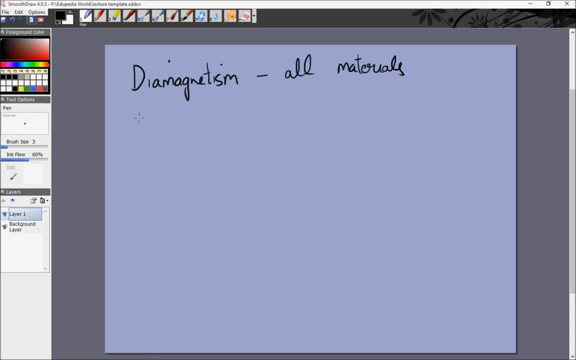 completely overwhelms the entire material, and that is what we are going to talk about in this video: an overshadow: the phenomena of diamagnetism. so first we'll see the phenomena of diamagnetism, which exists in all materials. now, here I'm in a little bit of a mind, because the phenomena of diamagnetism is due to a 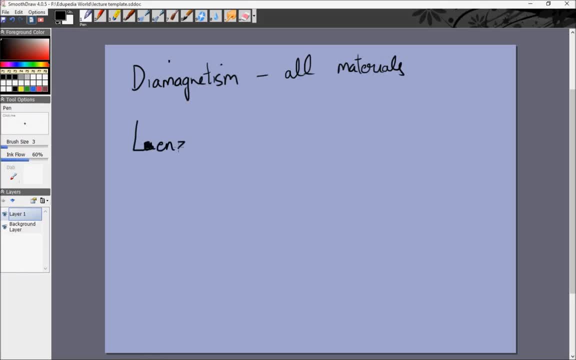 particular law called Lenz's law. right and Lenz's law we'll study in great detail a little bit later, when we move on to electromagnetic induction. that will be when we will actually combine. all of the elements that we have is just given in the form of electrostatics. 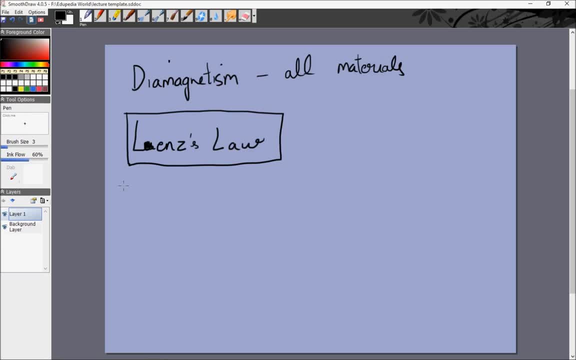 electrodynamics, magnetostatics and magneto dynamics, which as soon as you join that, it is called electrodynamics. so that's when we'll study Lenz's law, but right now I'm just going to write lenses law and not going to prove it. I'm 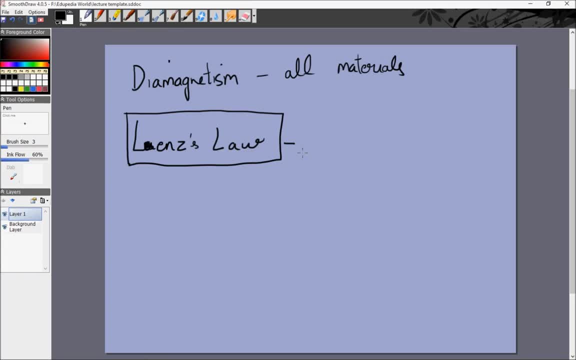 not going to really explain it that much as well, and I hope you will trust me that once we reach electromagnetic induction, I will completely explain Lenz's law to you. so Lenz's law states that the magnetic field due to- I'll just write B- due to Bол. 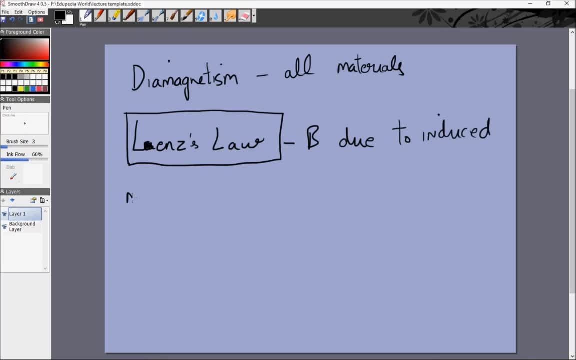 induced magnetic moment opposes the original field. Now let me just start by a parallel with electrostatics again. So when you have a certain material in which the molecules are not polar at all, what is a molecule or an atom which might not be polar at all? 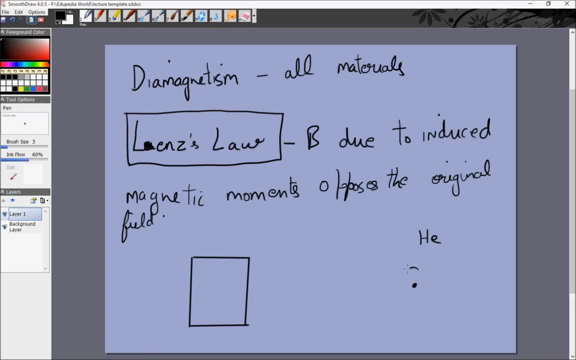 The helium atom is a good idea. right, You have one single nucleus and electrons moving around it, and when you apply an electric field in this direction- the nucleus, which is positively charged, and this which is called the electron cloud, which is negatively charged- initially the nucleus would have been at the center of the electron cloud. 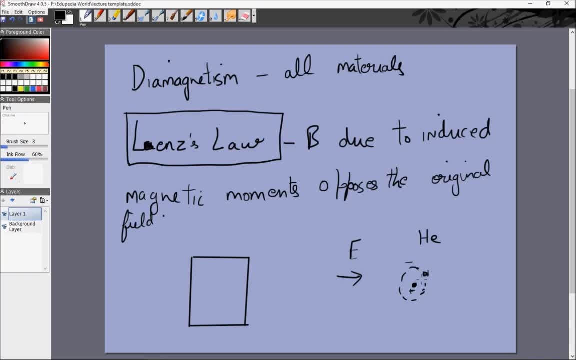 But because of this the electron cloud might shift a little bit towards the left and the nucleus might shift a little bit towards the right. Of course, the movement of the electron cloud will be much greater than the movement of the nucleus, So we then end up with an electric dipole moment in this direction, right. 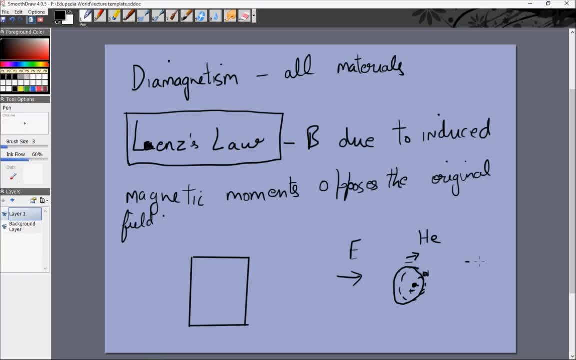 Because the negative charge moves towards the left and the positive charge moves towards the right. So this is the direction of the dipole. So this is something we have seen earlier, that even in a completely non-polar atom or molecule, when we put an electric field, 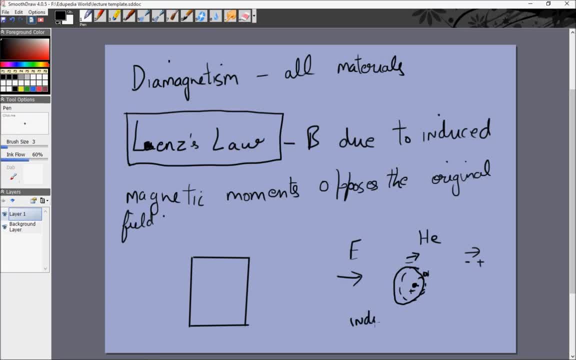 there is some induced dipole moment And actually, even if the molecule is originally polar, the polarity will shift a little bit because of this electric field. it will change a little bit and that change can be taken to be the induced part and the original value can be taken to be the original part. 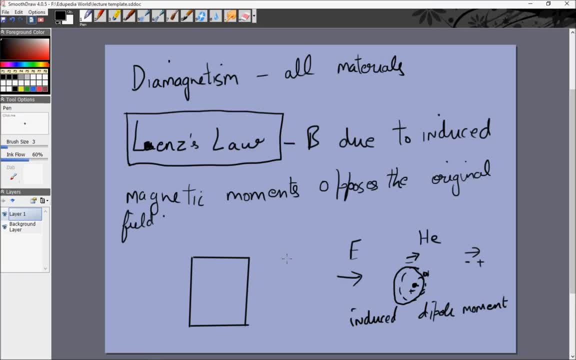 So in any material if you put an electric field there will be an induced dipole moment. Similarly- I will not explain this much right now, We will look at it later- in Lenz's law, But any material if you put it in a magnetic field. 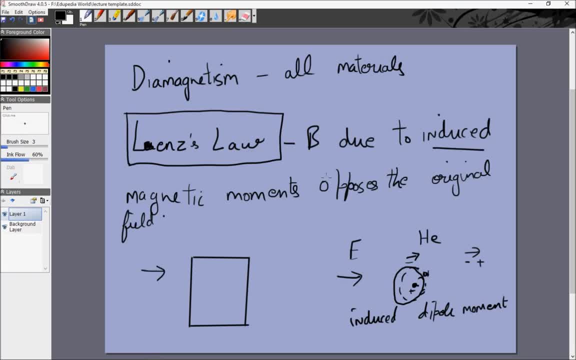 every atom, every molecule will experience an induced magnetic moment. Right Now, what does the induced dipole moment do? If this is the total material it ends up creating- sorry, a negatively charged surface here and a positively charged surface here. 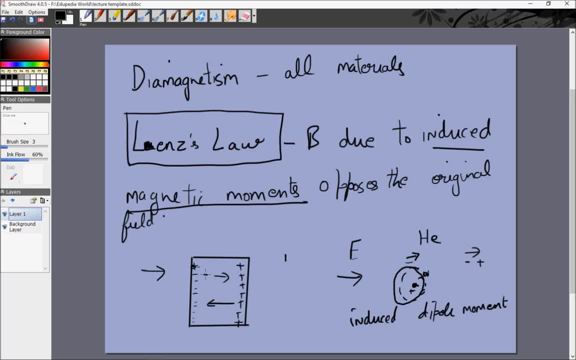 And it ends up creating an electric field in the opposite direction to this Right. That's what we have seen previously. So, similarly, Lenz's law states that the magnetic field due to these induced magnetic moments is opposite to the original field. 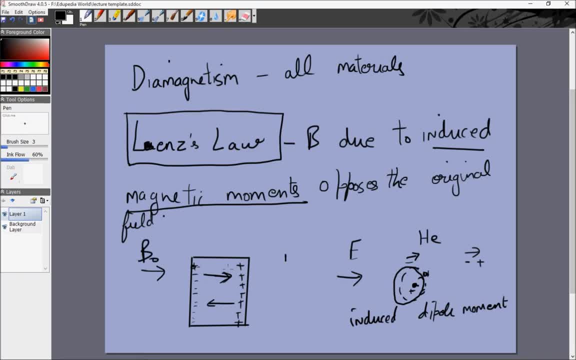 So pretty much the same thing happens. if we apply a magnetic field B0, then that magnetic field B0 exists. then due to the induced dipole, induced magnetic dipole moments, there is a magnetic field B in the opposite direction and let's say this is called Bi, B induced. 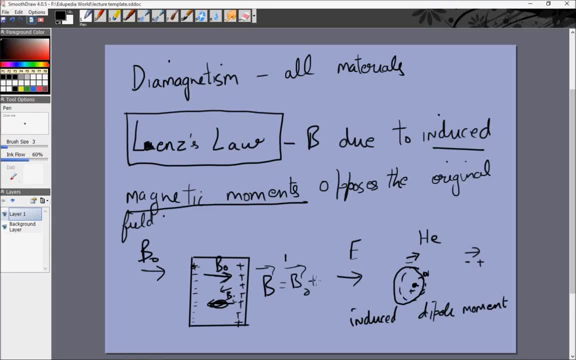 then the net magnetic field is equal to the vector sum of B0 plus Bi, or the mod of B is equal to B0 minus Bi. Right, So this happens in every material, whether the molecules and atoms are polar or non-polar. 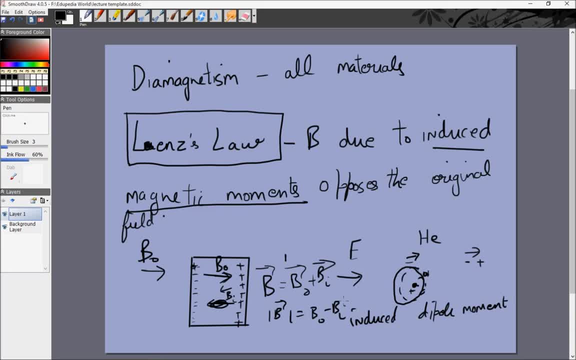 whenever you put them in a magnetic field, there will be a certain amount of induced dipole moment, and that induced dipole moment introduces its own magnetic field, which is opposite to the original field, just like in the case of electrostatics. So right now we've completely mirrored electrostatics. 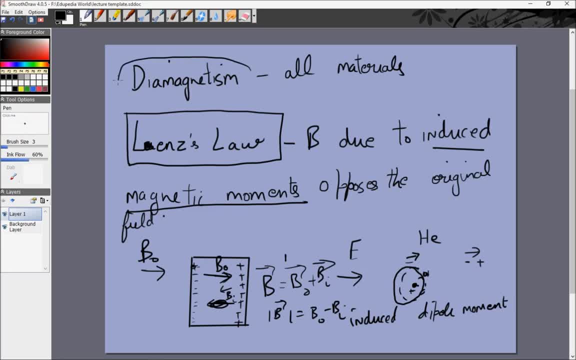 and this process is called diamagnetism, and the materials which exhibit this, and only this, are called diamagnets. So right, so every material shows this phenomena, but in most materials this is not observable, because paramagnetism or ferromagnetism dominate. 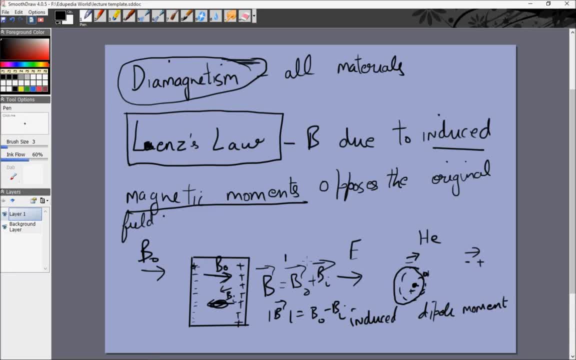 So the materials in which you can see this are called diamagnets, and a nice way of showing diamagnets in terms of electric field lines is this: If this is a diamagnetic material, electric field lines generally might be like this Right, let's say, in a certain region. 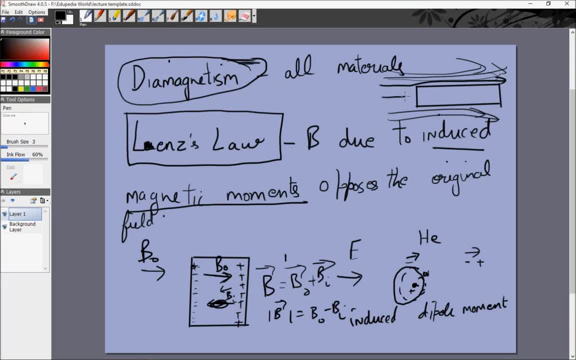 Then they'll become like this, That is, the density of electric field lines will reduce near the diamagnet. Right here there will be a large density of electric magnetic field lines and we've seen just like in electric field lines and magnetic field lines. 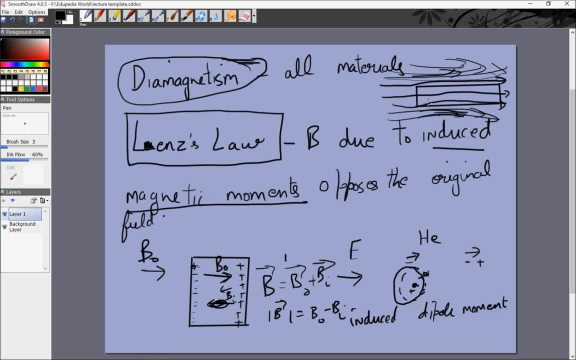 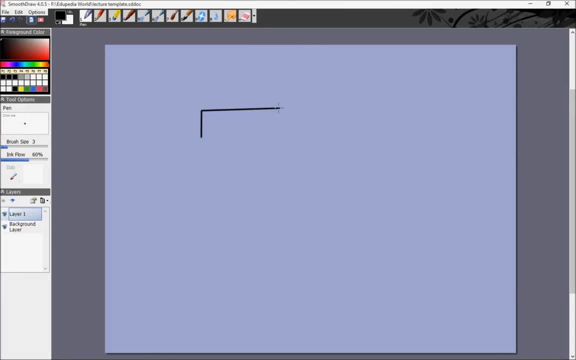 where the larger number of field lines per square area, per unit area, the greater the magnetic field. So I'll just draw this figure better. I'm not satisfied with this. So this is the diamagnet. Then the magnetic field will be influenced like this: 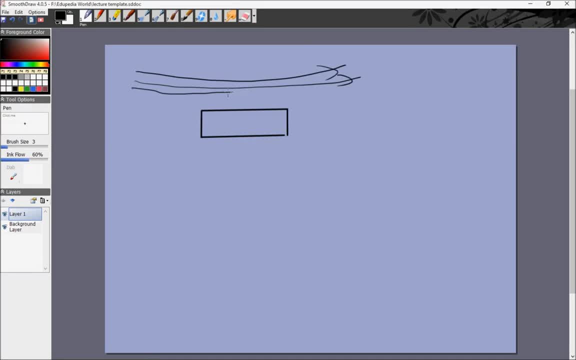 If this was the magnetic field originally- and this is the way it kept going, then now, when it reaches the diamagnet, it might become something like this: Only two lines flowing And then, sorry again, many, many lines. Yeah right. 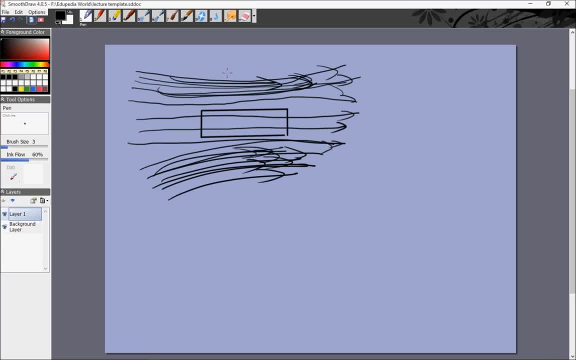 So this is the way you can see it. There will be magnetic field lines all over, and when you introduce the diamagnet, some magnetic field lines will even start repelling, like this, and there will be few number of magnetic field lines within this diamagnet. 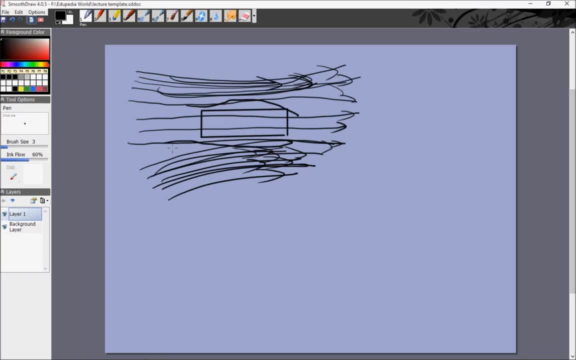 That is a manifestation of the fact that the net magnetic field is smaller than the original magnetic field. So what is the property of diamagnets? They tend to align antiparallel to the magnetic field, Right, that is, if we introduce a magnetic field. 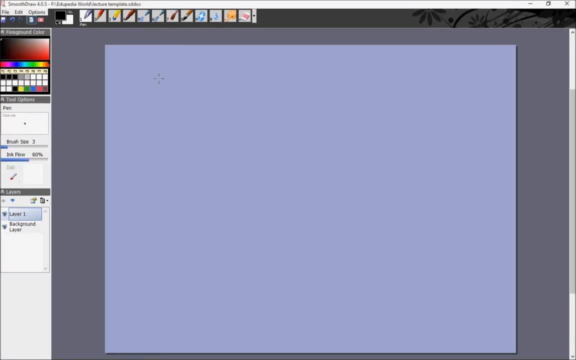 the net magnetic field within that material will be smaller than the introduced magnetic field. Now let's look at the more interesting cases. The first one would be paramagnets. Now, what happens in paramagnets is paramagnetic materials. first of all are those: 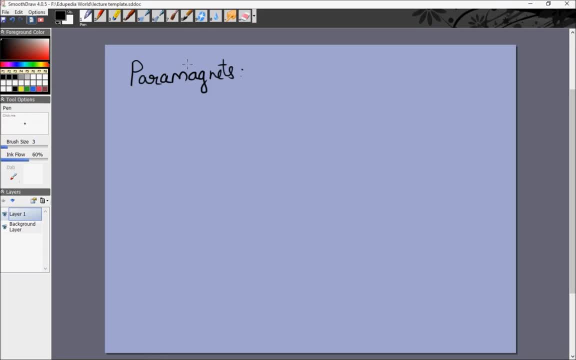 in which the atoms or molecules already have a dipole moment. So already polar, Right now, for all materials, polar or non-polar, diamagnetic materials, paramagnetism exists. Paramagnetism exists for only molecules which have their own magnetic dipole moment. 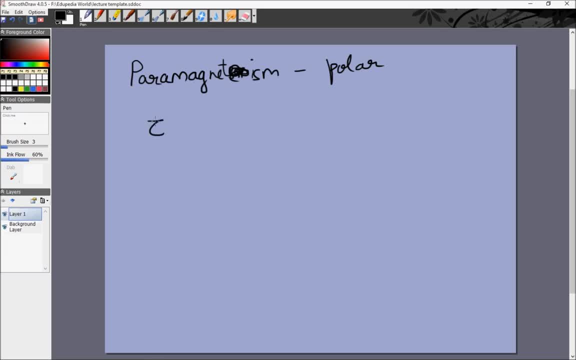 Right. so what happens in this case is the torque is equal to mu. cross b tries to align all the dipoles parallel to the dipole moment, Right? so what happens is, if initially dipoles were in random directions, then once you apply a magnetic field, 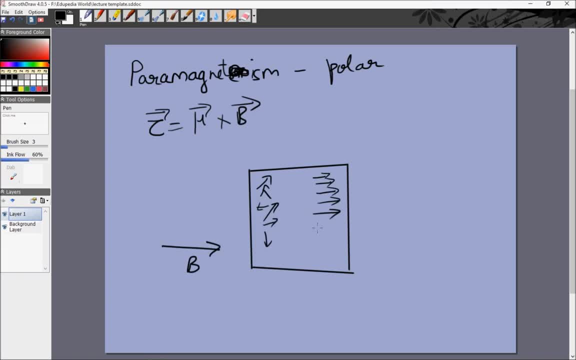 the dipole will align like this. Again, it's not necessarily that they will be completely aligned, but they will be aligned like this Right now. in this case, the net magnetic field will increase. that means this B- let's call this B0,. 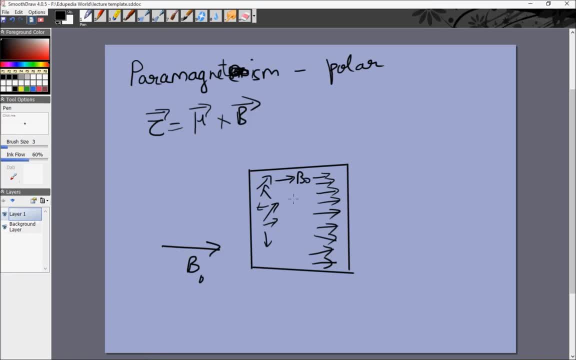 and let's call the magnetic field induced due to these dipoles B Bi, then that Bi will also be in the same direction and the net magnetic field will be greater than B0.. Now why does this happen? We didn't see this in the case of electrostatics. 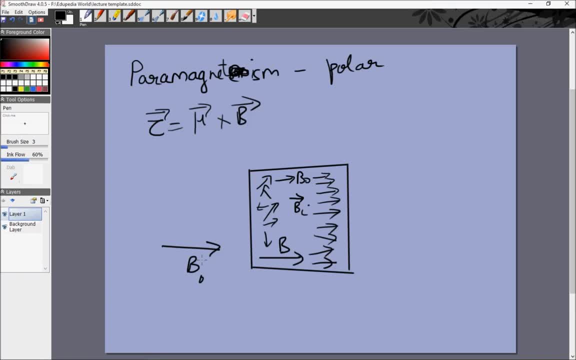 and that's because there's a very big difference between an electric dipole and a magnetic dipole which we've seen previously. An electric dipole might be like this: minus plus, pointing in this direction. magnetic dipole like this, this side is near you. 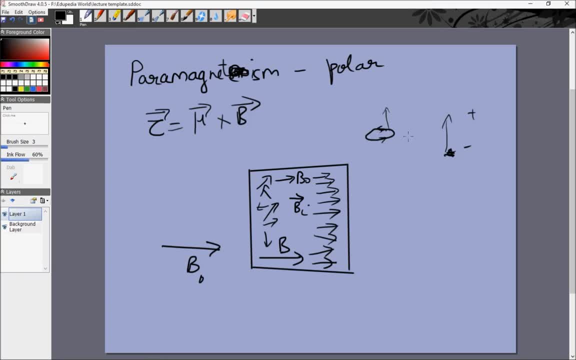 this side is away from you. so again in the upward direction, Right, the difference is. outside they're pretty much the same. these are the field lines, But inside, because electric field lines start and end at a point within this dipole. 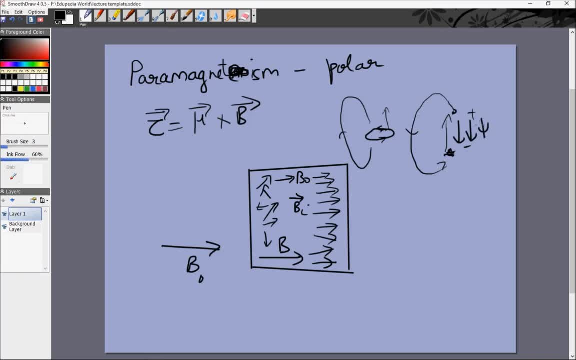 electric field lines are in this direction that is opposite to the dipole moment. However, here they go like this: Right, because these magnetic field lines are always in complete circles. Right, and you can just see that directly when you curl your fingers around this. 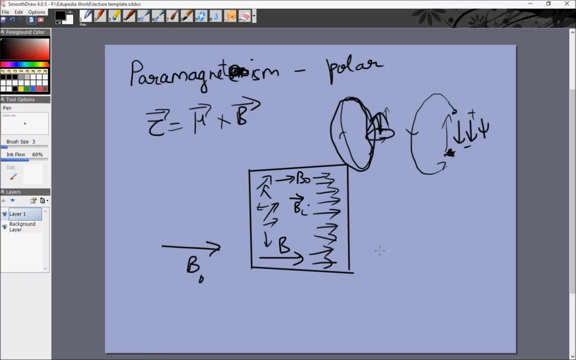 the magnetic field is in the upward direction. So when placed in a magnetic field, the magnetic field due to a dipole is in the direction of the dipole, But the electric field due to an electric dipole is opposite to the dipole moment. 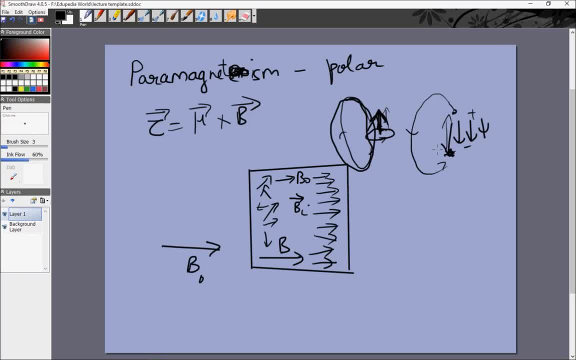 Right, and this is a big, big difference between an electric dipole and a magnetic dipole, and this difference is the only reason paramagnetism exists. Right, so the net magnetic field will be the sum, as always, of B0 and Bi. 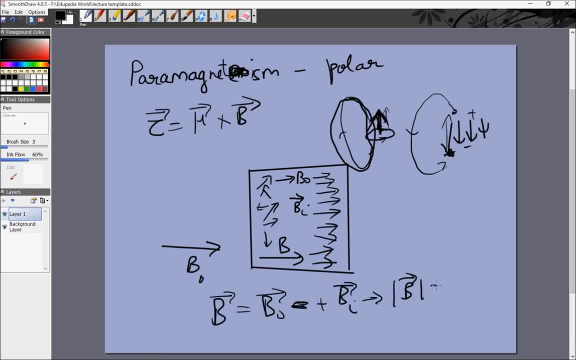 and in this case the magnitude will be B0 plus Bi Right. so diamagnetism: the net magnetic field is smaller than the original induced magnetic field. Paramagnetism: the net magnetism is greater than the original magnetic field. Why? Because in diamagnetism the magnetic field of induced dipole moments is opposite to the original magnetic field. where Lenz's law? whereas in paramagnetism there is no induced dipole moment, There is just the original dipole. there is a small induced dipole moment which causes diamagnetism, but the molecules are already polar, so there is already a big, big dipole moment. Generally, the induced dipole moment is much smaller than the original dipole moment, so that's why diamagnetism is not really observable. 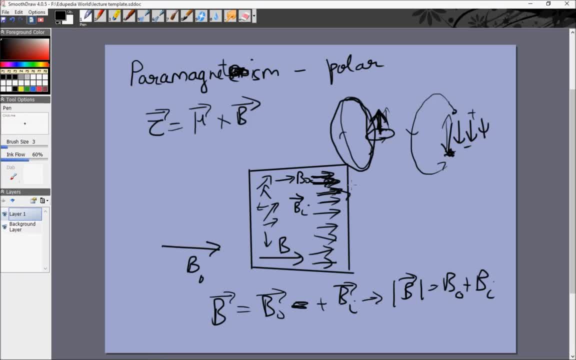 in paramagnetism, though it exists. So the magnetic field due to these dipoles, they increase the magnetic field net because their magnetic field is in the same direction as B0 and that's why the net magnetic field is greater, Right? so 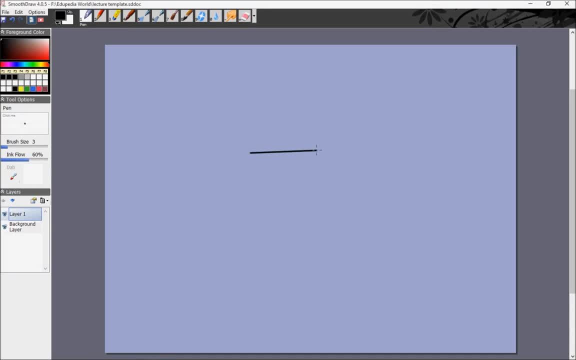 paramagnets. in terms of magnetic field lines would probably be shown something like this: If these were the electric field lines, then they would really start to have a greater density within the magnets. So this would be something like how the electric magnetic field lines would look. The density would be greater within the paramagnet. So it sort of has the tendency of absorbing magnetic field from the other side, even though it doesn't really do that to increase the magnetic field within it. Now, ferromagnets are essentially an extreme. 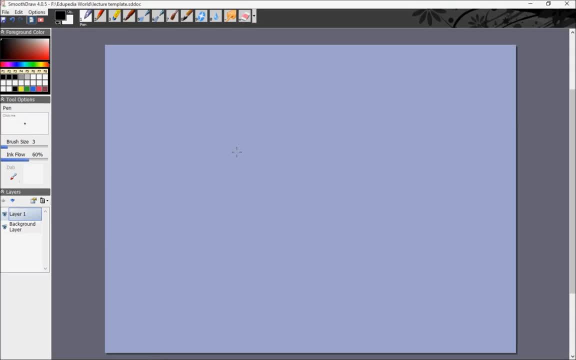 version of paramagnets. In them the magnetic field is also greater than the induced magnetic field, but it's greater by factors of thousands or tens of thousands because the original magnetic field of the material itself, not the magnetic field we put it in. but 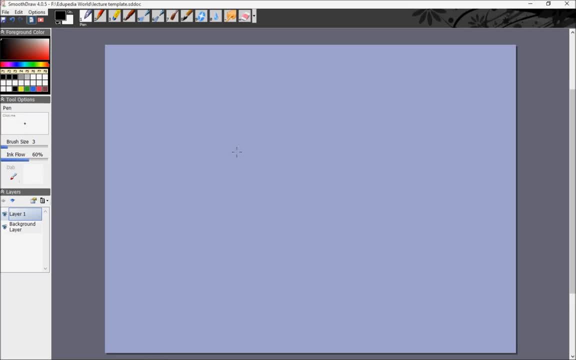 Bi is actually very, very large. So the property of ferromagnets is that sometimes because of something called exchange coupling- this is not in your course, but you will study this in advanced quantum mechanics- but because of this phenomena in ferromagnets. atoms have a tendency to align themselves parallel to each other, even when there is no magnetic field present Right. But generally a complete material does not align itself in the same direction. It consists of what are called domains. So ferromagnetic materials are materials like iron. 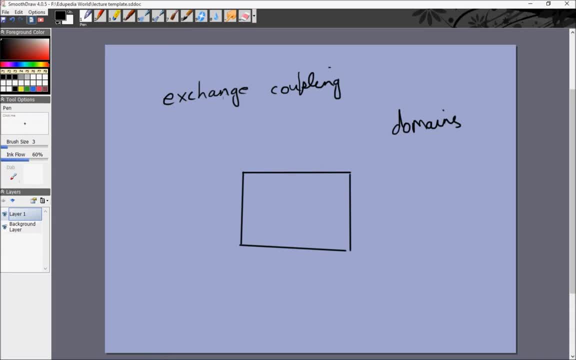 and those materials. even when there is no magnetic field, when they are just stationary, they are divided into many domains. So if this is a cubical block, it would be something like this: Right, These will be different domains, I don't need to draw all of them. 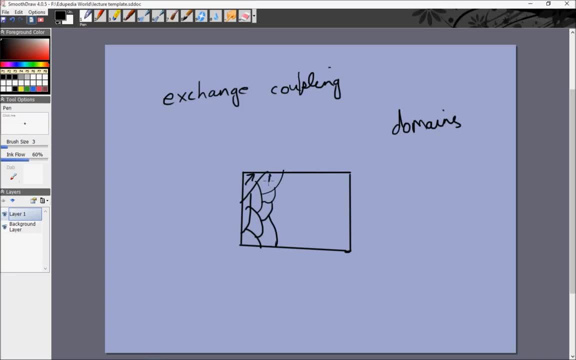 This domain will have a magnetic dipole moment in this direction. This domain will have a magnetic dipole moment in this direction. This domain will have a magnetic moment in this direction, this direction, this direction, So, even though the atoms align themselves parallel to each other, 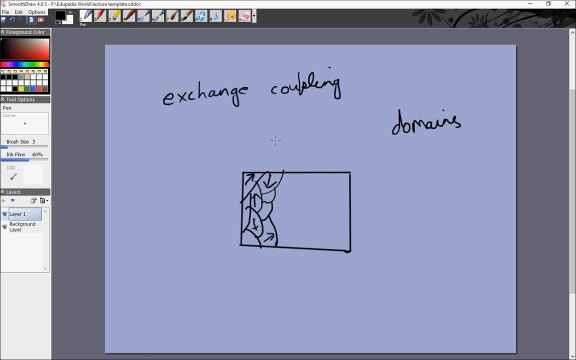 all domains are not parallel, But neighbouring atoms end up aligning themselves parallel to each other. So these two atoms will be parallel to each other in this direction, But these two atoms will actually not be parallel. So this is the standard state of ferromagnetic materials. 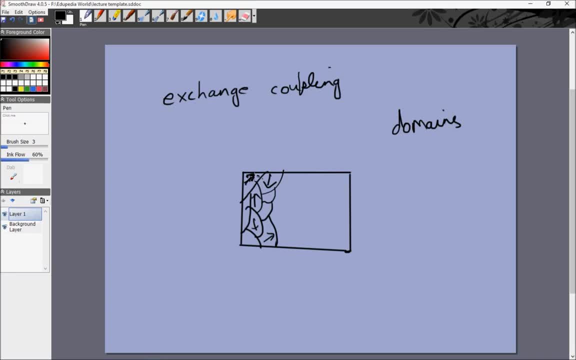 You have these big domains consisting of millions and millions of atoms and molecules, and they all point in the same direction. Now, when you introduce a magnetic field within a ferromagnet, then the net magnetic field increases due to two processes. One is domain growing. 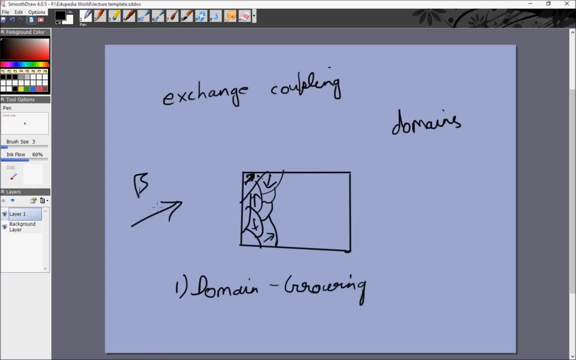 and all that happens is- let's take this to be completely horizontal- then there will be some domains which will have completely horizontal or nearly completely horizontal magnetic moment. So, because of this magnetic field, the nearby these, for example molecules or atoms- will also. 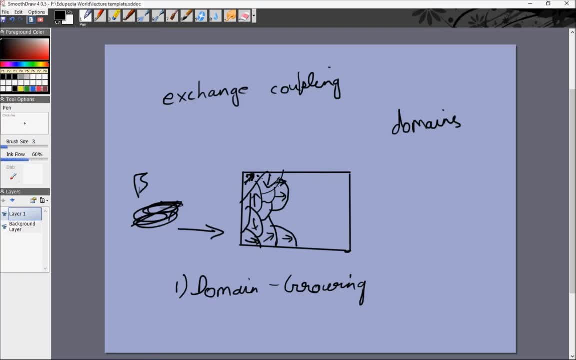 switch their magnetic moment towards the right Right. So what happens is these domains start growing and these other domains start shrinking. So eventually, what will happen is it will be something like this: These would be the domains pointing in this direction and these would be the smaller domains. 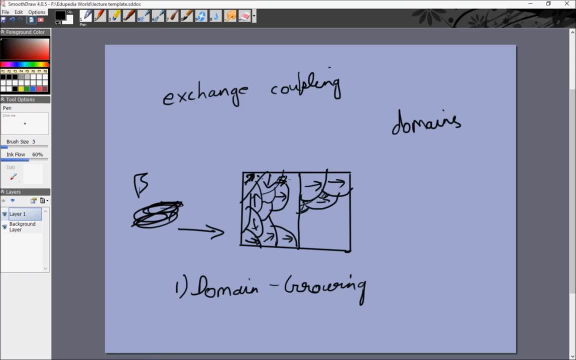 Right, Because all these atoms would start pointing in this direction by, again, the phenomenon of exchange coupling. So one is the domains which are in the direction of magnetic field start growing and the other starts shrinking, and the other is called domain alignment And, as the name suggests, 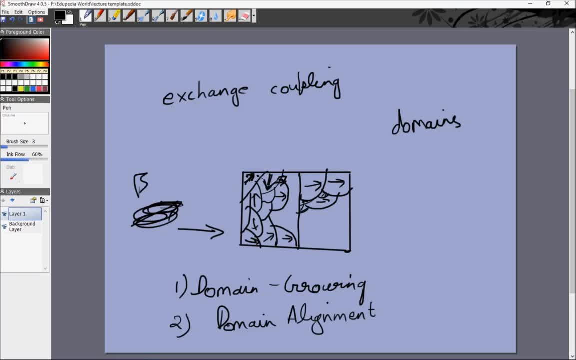 it is about aligning the domains, So the domains which have a magnetic moment in this direction. sometimes the complete domain will flip and switch towards this direction. So instead of these domains increasing its size, we are actually getting the other domains and pointing them in the direction of magnetic field as well. 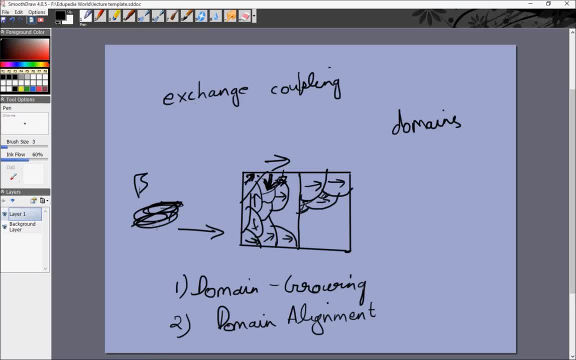 How this process actually occurs is not in your course. In fact, even I don't know it properly, because it is in very high quantum mechanics that you actually study this stuff. Right? So these are the two processes, the domains parallel to the magnetic field.